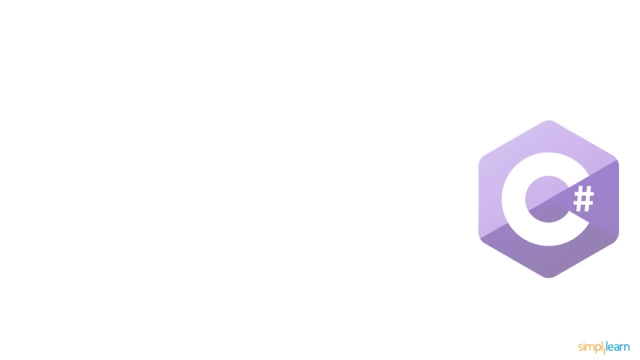 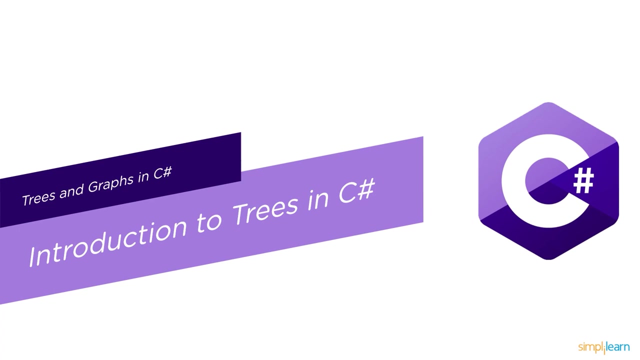 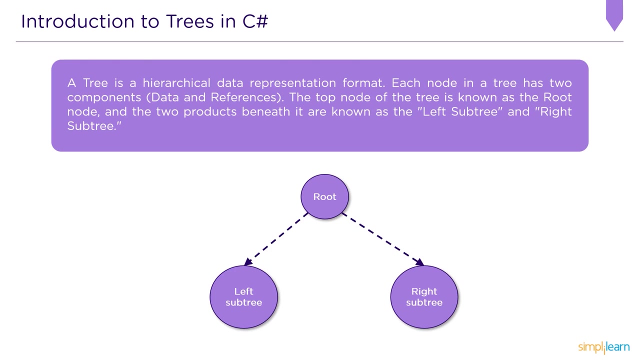 then solved efficiently using this model. After understanding the importance of tree and graph data structure, now let us understand the tree data structure. to proceed with the introduction, The tree is an hierarchical data representation format. It is used to represent the tree as a whole or as a whole. Each node in a tree has two components: data. 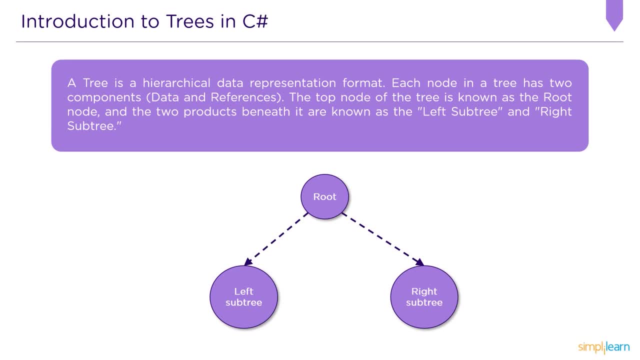 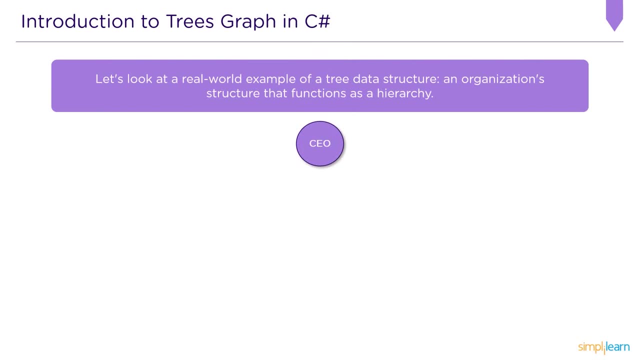 and references. The top node of the tree is known as the root node, and the two products beneath are known as the left subtree and right subtree. Also, they are called as children. Let's look at the real world example of a tree. data structure, An organization structure. 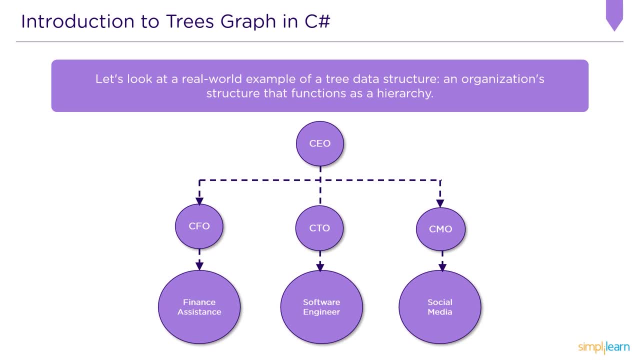 that functions as an hierarchy. So here's an example of how an organization where the CEO works. Then we have children that are CEO, and CFO, which are the chief financial officer and chief technical officer, And we also have CMO, that is, chief marketing officer. 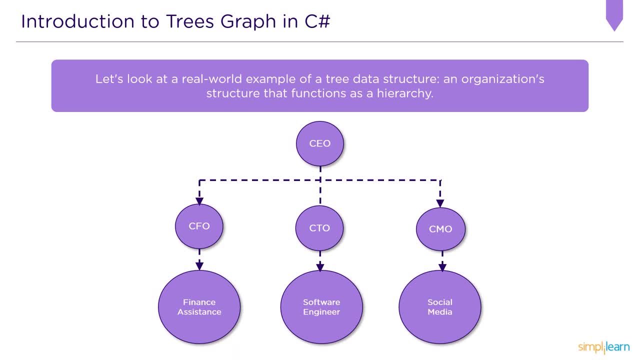 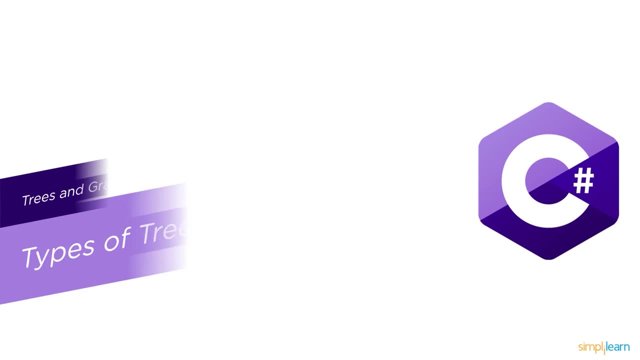 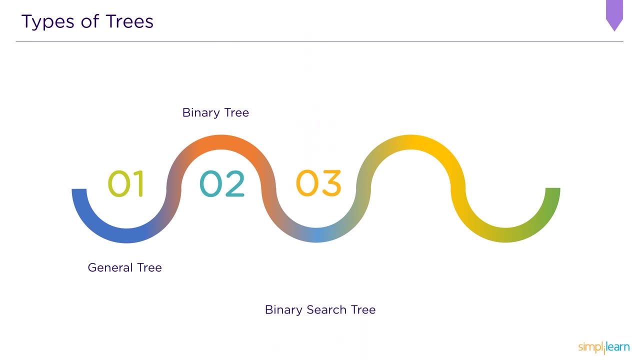 Then we have children of CFO as financial assistance and CTO as software engineering, And finally we have social media. Following this tutorial, we will look at the various types of trees. So there are only five types of trees: The general tree, the binary tree, the binary search tree, the ABL tree and the red black tree, which is a final or fifth type of tree. 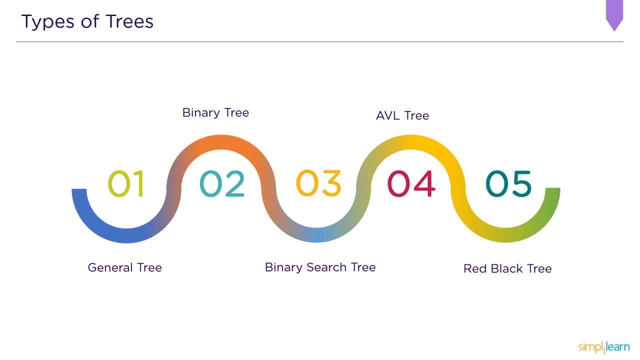 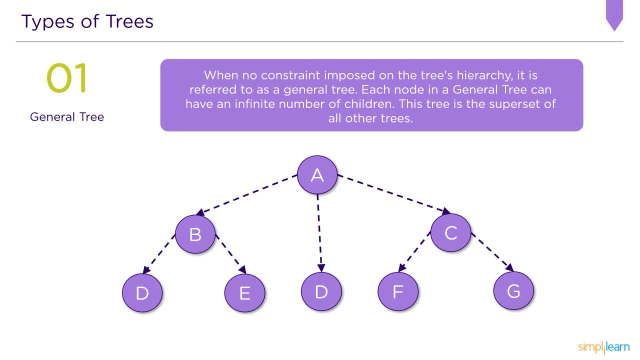 Let's look at all of these different types of trees by defining them all. We have the general tree first. When no constraint is imposed on tree's hierarchy, it is referred to as general tree. Each node in the general tree can have an infinite number of children. 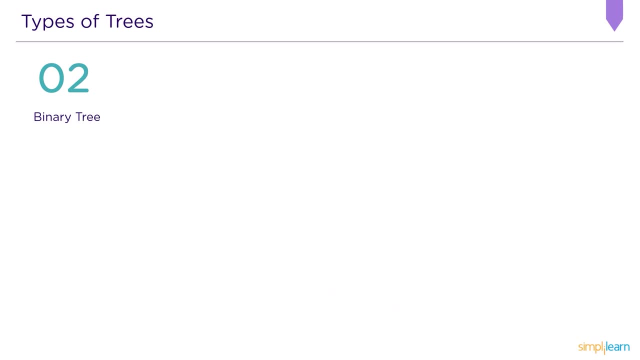 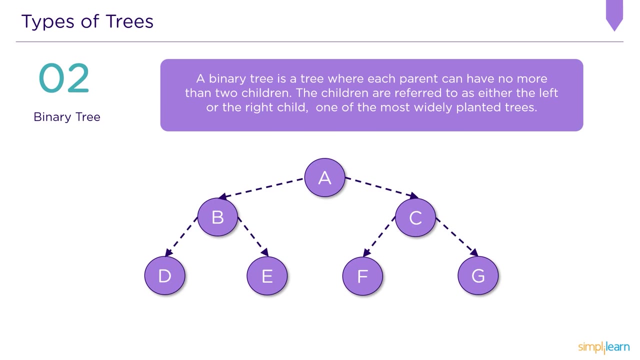 This tree is a superset of all other trees. We also have a binary tree. A binary tree is a tree where each parent can have no more than two children. The children are referred to as either the left or right child. one of the most widely planted trees. 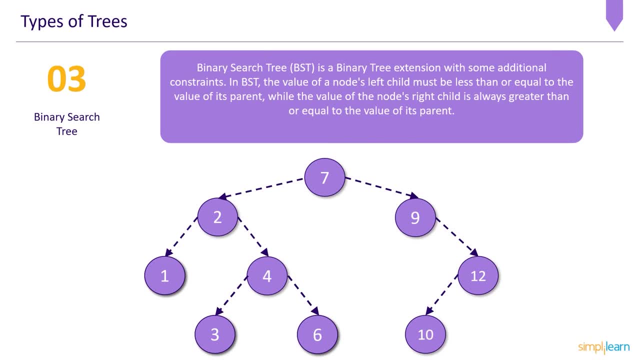 The binary search tree is the next type of tree. Binary search tree is a binary tree extension with some additional constraints. In BST or binary search tree, the values of a node left child must be less than or equal. The value of a node's right child must be equal to the value of its parent. 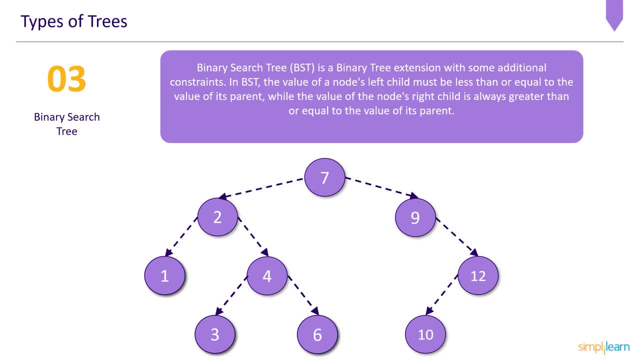 While the value of a node's right child is always greater than or equal to the value of its parent, The binary search tree property makes it suitable for searching operations because we can determine whether the value will be in the left or in the right subtree at each node. 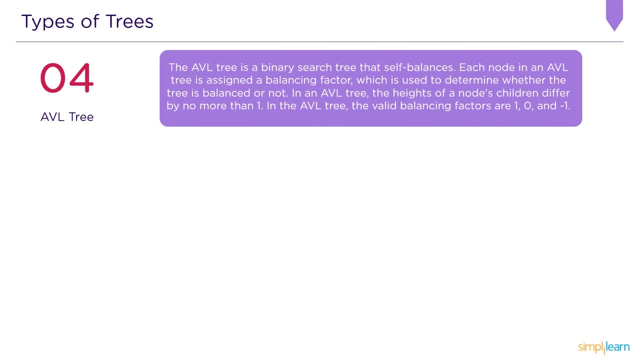 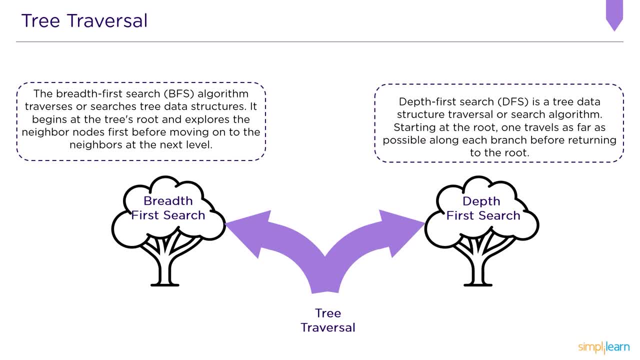 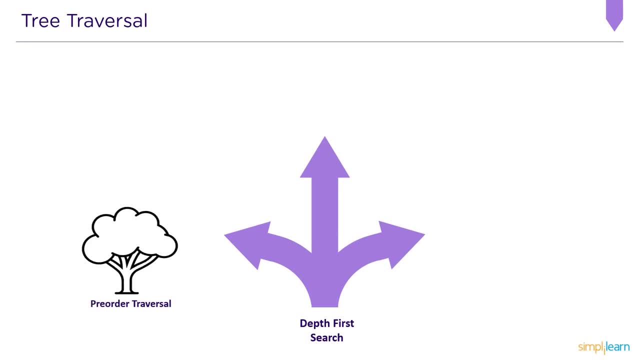 as possible, along with branch. before returning to the root, that first search tree traversal has been classified into three modes of traversals, so we have pre-order traversal, in order traversal and post order traversal. let us try to define all these traversal in greater detail, for example, in pre-order. 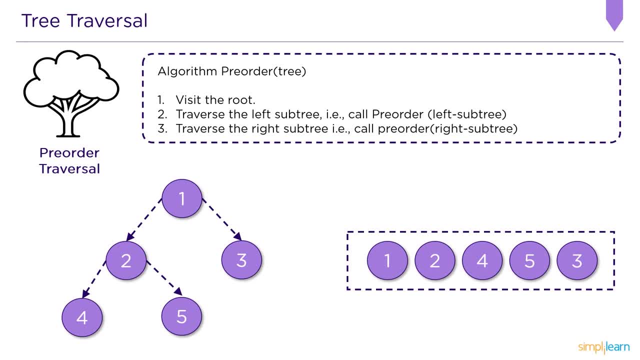 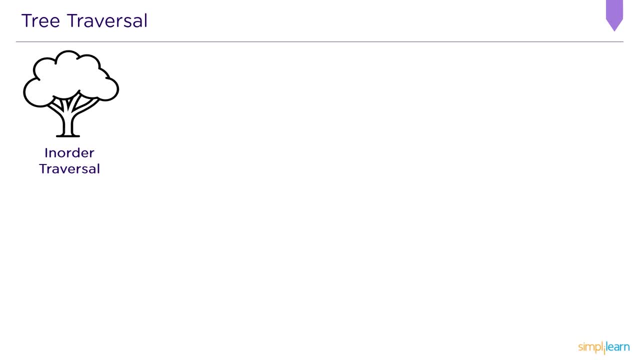 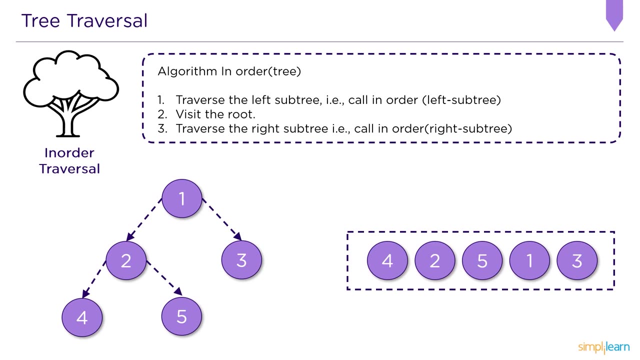 traversal, we first visit the root node, then the left subtree and finally in the right subtree. for a better understanding, consider the following example of pre-order traversal. next we have the in order traversal, which means that in this type of traversal we first traverse the left subtree, then the root node and 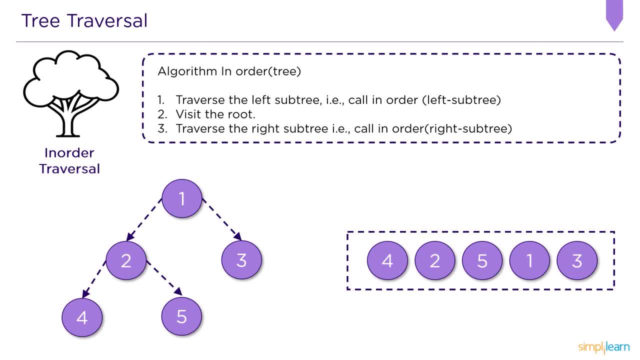 finally the right subtree. so for a better understanding, here is an example for in order traversal. finally, we have the post order traversal. in post order, we first traverse the left subtree, then the right subtree and finally the root node. for a better understanding, here is an example of post order. 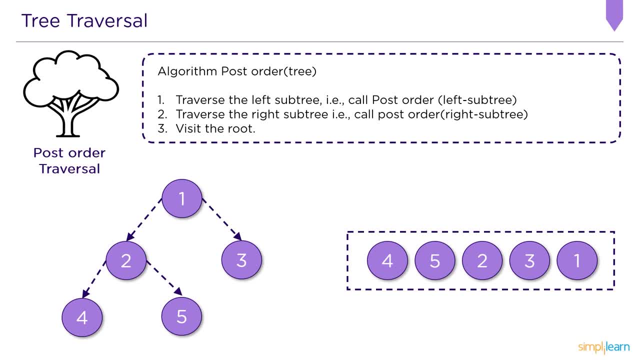 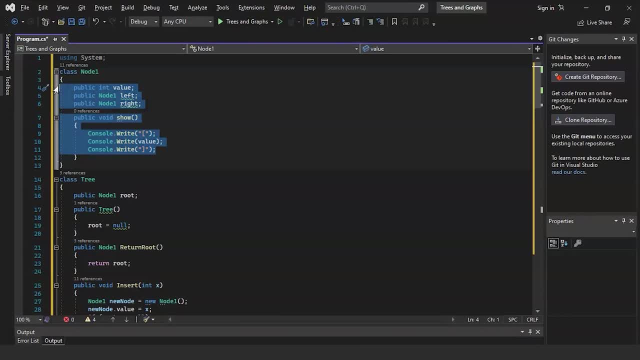 traversal. let us look at code demonstration for tree traversal with pre-order in order and post order. in this program we first define a tree node as node 1, with values left and right, and then we define a show function to display all the tree traversals, and in this function we defined a value in 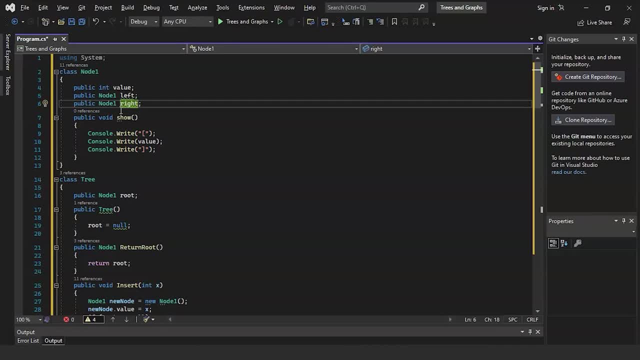 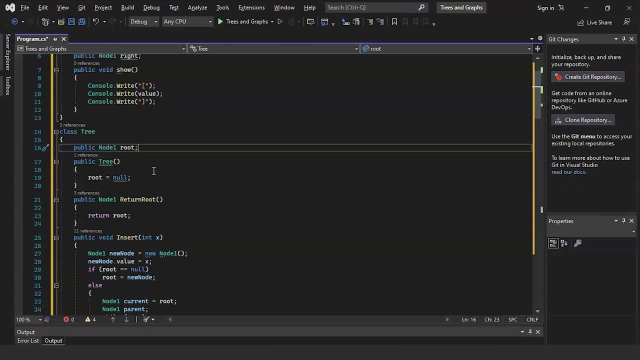 square brackets. following that, we created a tree in which the root node is null initially. then we have a function, namely return root, where we will return the root value, and finally we have the insert function. and finally we have the insert function, in which we create a new 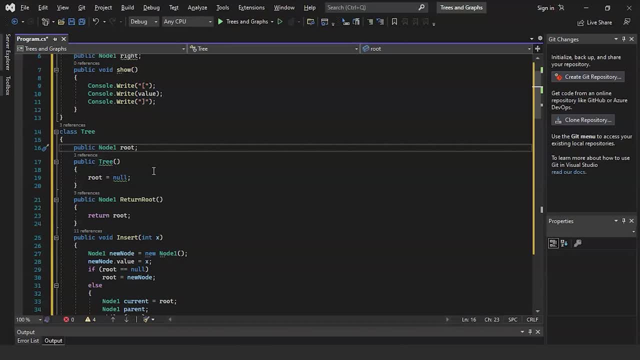 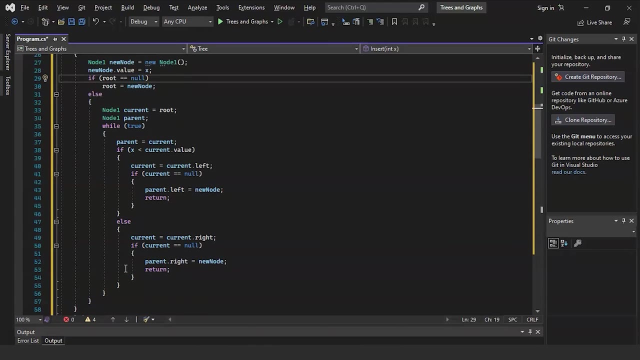 node and insert X value to that new node. after that we have a condition that says if the root node is null, we will assign the new node as the root node. otherwise the root node will be assigned as the current node, defining the parent node. following that, we assign the current node to the parent node with the. 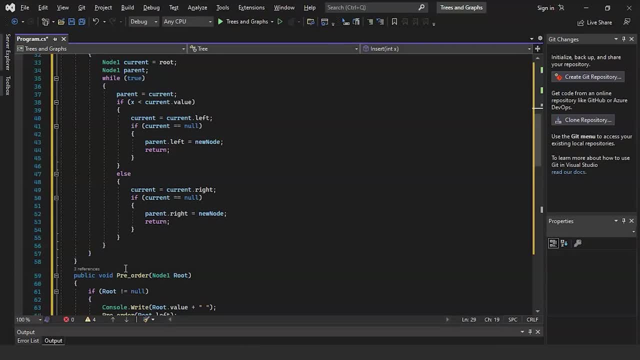 condition that if the assigned value X is less than the left node, we assign that value to the left node, and if the left node is null, we will assign a new node to that left node and the right node. if the assigned value X is greater than the left node, we assign that value to the left node, and if the left node is. 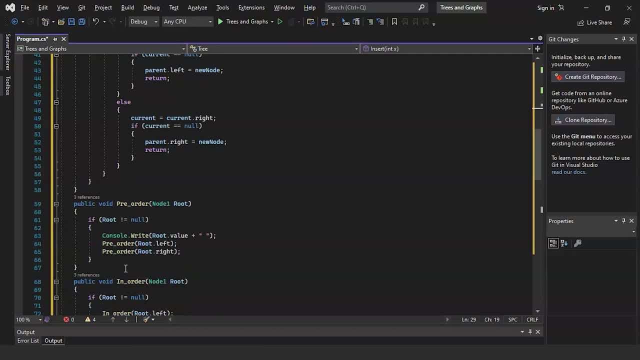 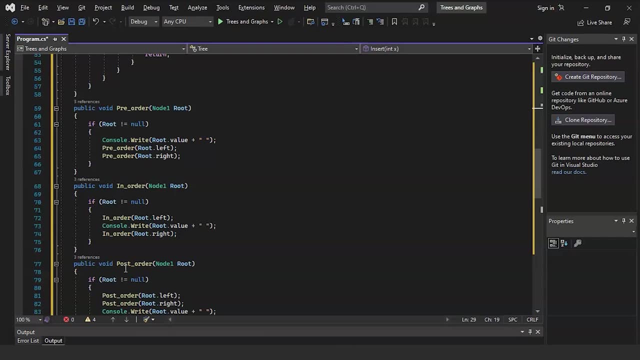 null, then we will assign a new node to the left node. now we will define all three tree traversals first. we'll have to do pre-order traversal, which means that if the root node isn't null, the first will give the root node and we will prefer to traverse first the 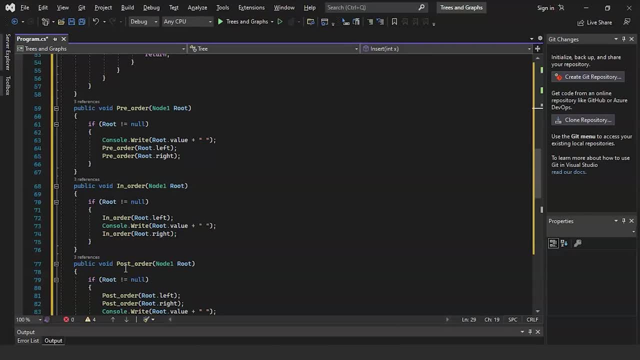 left node, then the right node. next, if the root node is not null, we will call to traverse the left tree, enter the root value and call pre-order to traverse the right tree. finally, in post order, we will call post order to traverse the first left and right tree and then assign the root value if the root is not null. 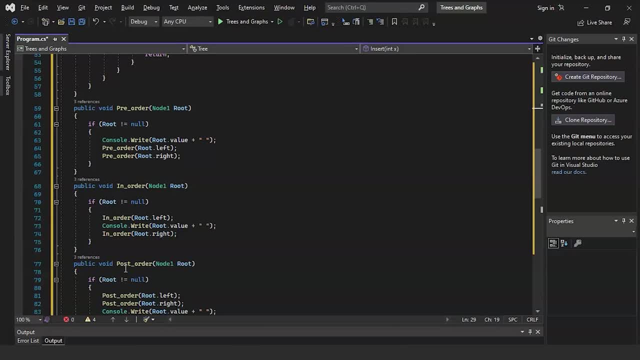 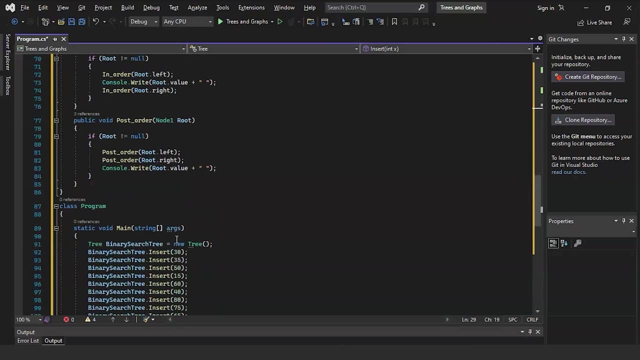 finally, we created a binary search tree in the main function. here we've provided the Boolean name for the root node. we shall now call it the insert function to insert all the values. finally, we will call the in order function to perform in order traversal, followed by the pre-order traversal, and. 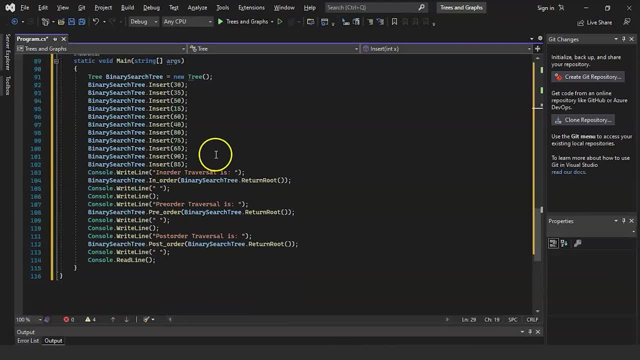 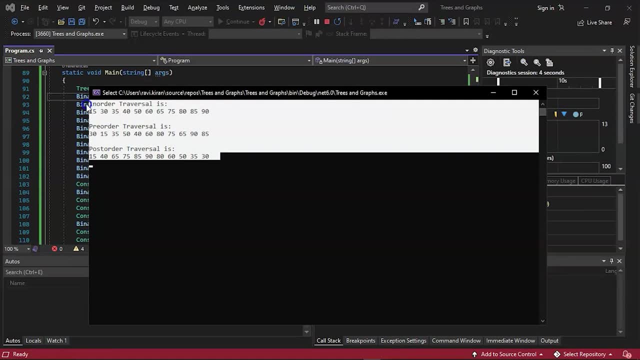 finally, we'll call post-order function to perform post-order traversal. now let's quickly try to execute the program and see the output. there you go. the program got successfully executed and we have all the three types of traversals in order traversal, pre-order traversal and post-order traversal. 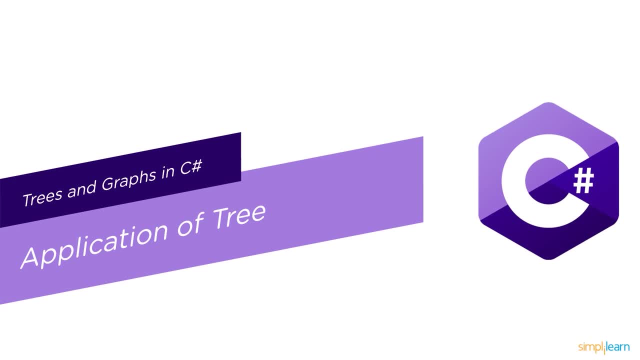 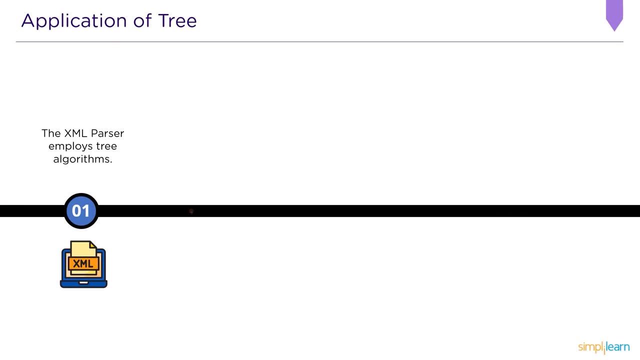 back to the slides now. the next topic is the applications of trees. we have five applications of tree data structures in c-sharp. the first application is the xml parser, which employs the three algorithms. the tree's second application is a decision-based algorithm based on the tree. 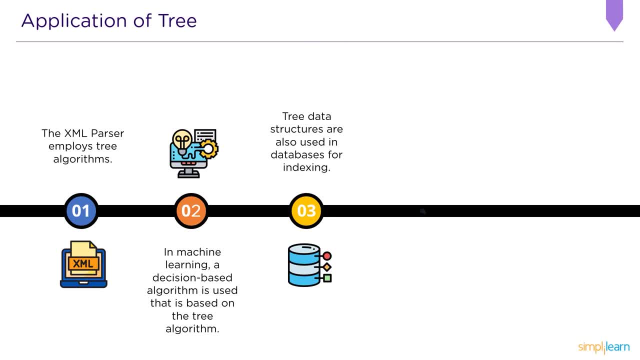 algorithm used in machine learning. the tree data structures are also used in databases for indexing. the third application of trees, the following use of a tree data structure: domain name servers also use tree data structures, that is dns. the fifth and final application of tree is file explorer mobility computer, any computer bst in computer graphics, after understanding the tree data. 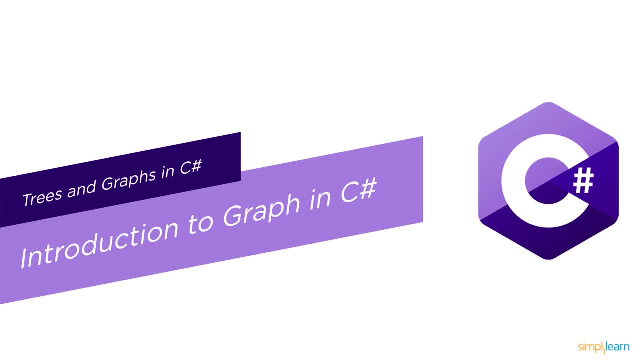 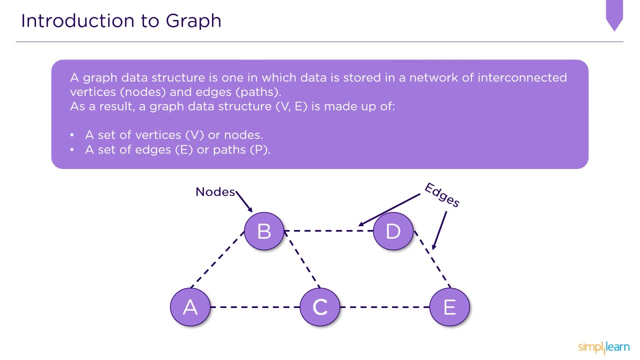 structure in c-sharp. we will now try to understand graph data structures. the graph data structure is one in which data is stored in a network of interconnected vertices, nodes and edges, also called as paths. as a result, a graph data structure that is made up of a tree data structure is a tree data structure that is made up of a tree data structure that is. 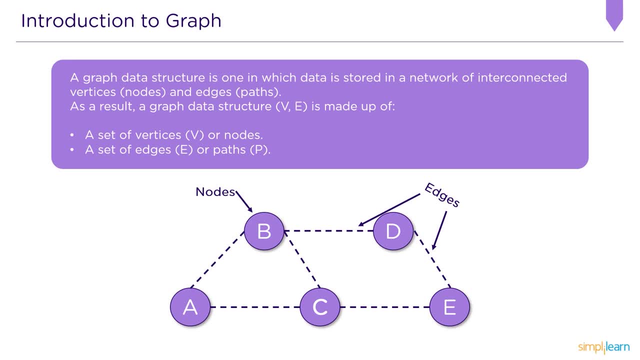 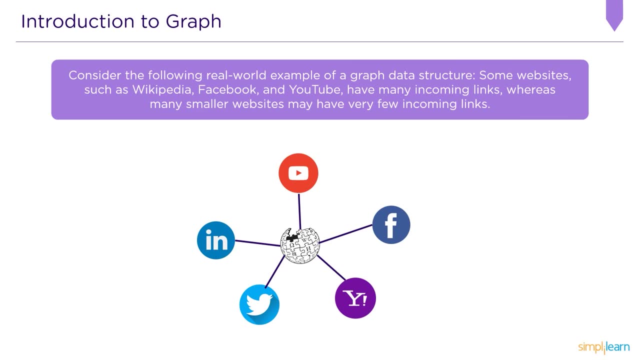 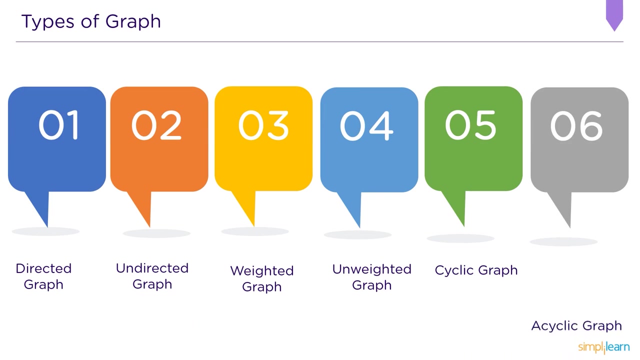 a set of vertices v and a set of edges referred as e or paths p. consider the following real world example of a graph data structure. some websites, such as wikipedia, facebook and youtube, have many incoming links, whereas many smaller websites may have very few incoming links. we will look at different types of graphs, so there are generally six types of graphs. 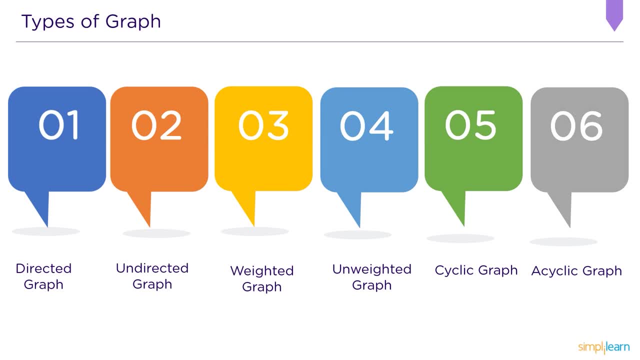 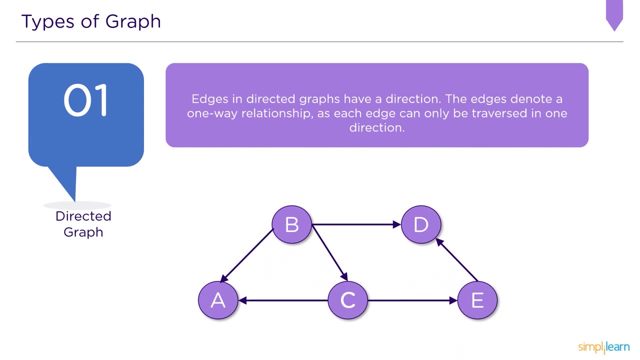 so first we will have directed graphs, next we have undirected graphs, weighted graphs, unweighted graphs and, finally, cyclic and acyclic graphs. let us try to comprehend all these graphs in greater depth. first and foremost, we have directed graph. edges in a directed graph have a direction. the edges denote one-way relationship, as each edge can only be traversed in one direction. 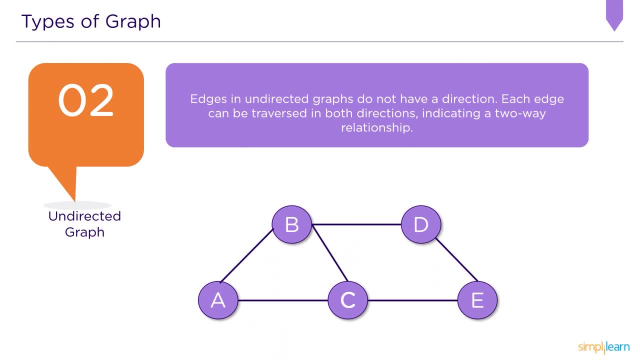 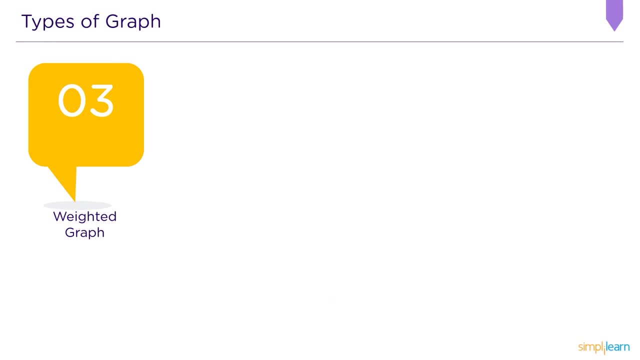 next, edges in undirected graphs do not have a direction. each edge can be traversed in both directions, indicating a two-way relationship. a weighted graph is defined as if the edges in your graph have weights, your graph is said to be weighted. next we have unweighted graph, which is defined as a graph that is said to: 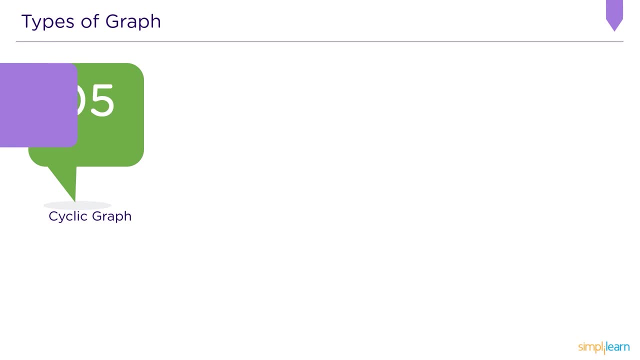 be unweighted if the edges do not have any weights after that. acyclic graph is a directed graph in which at least one node has a path back to itself. the last type of graph is an acyclic graph defined. an acyclic graph is a directed graph with no cycles, meaning that 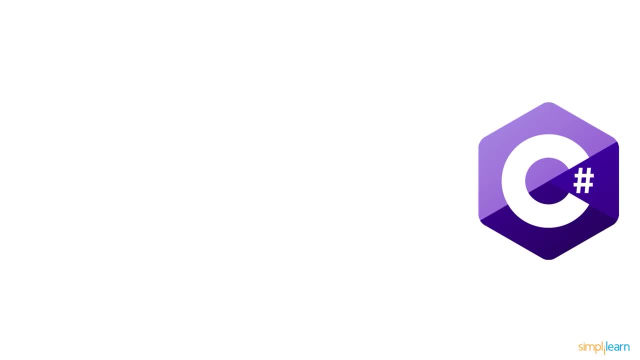 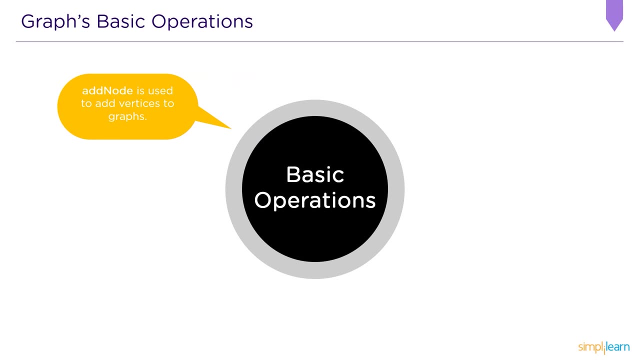 no note can be traversed back to itself. In this tutorial we will see some basic operations performed on graphs, after learning about various graph data structures. So first we have the addNode operation, which is used to add vertices to graphs. Next operation we did in the graph was to removeNode. defined as removeNode removes graph. 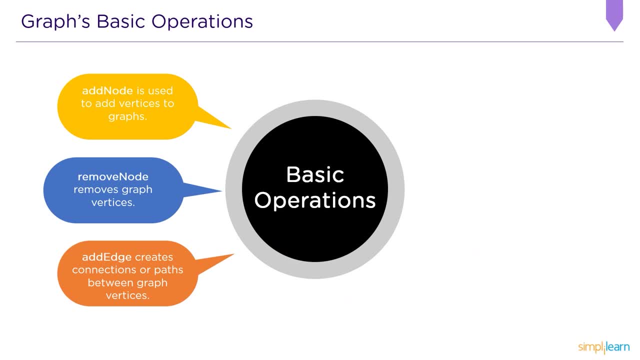 vertices. The third operation is the addEdgeState, which establishes connections or paths between graph vertices. The fourth operation is removeEdge, which is a function that removes connections or paths between vertices and graphs, Following that perform a check operation to see if a graph contains a specific value. 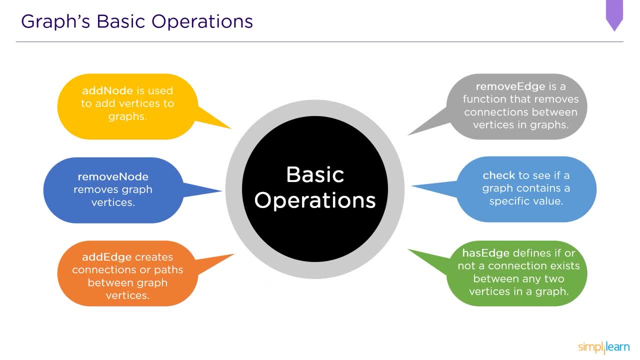 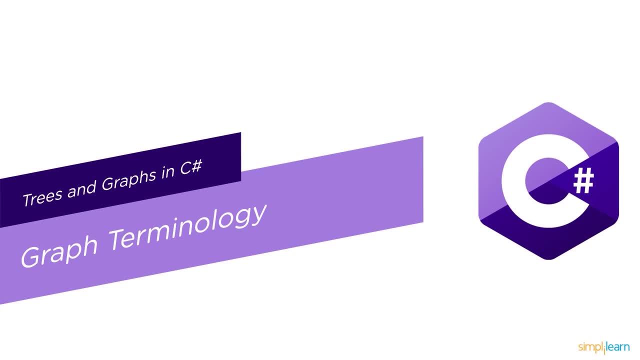 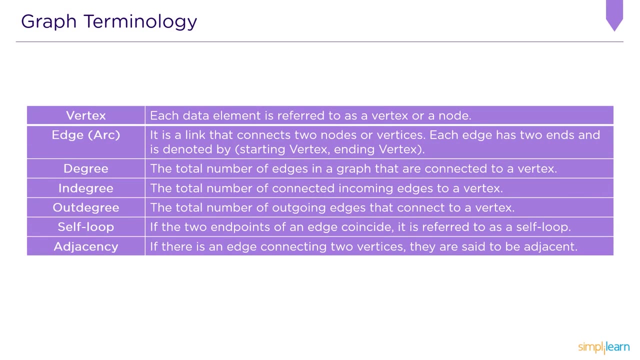 The sixth and final operation carried out in the graph has edges defined whether or not there is a connection or path between any two vertices in a graph. After understanding some basic graph operations, we will look at graph terminology First. a vertex is defined as a vertex, or node is a name given to each data element. 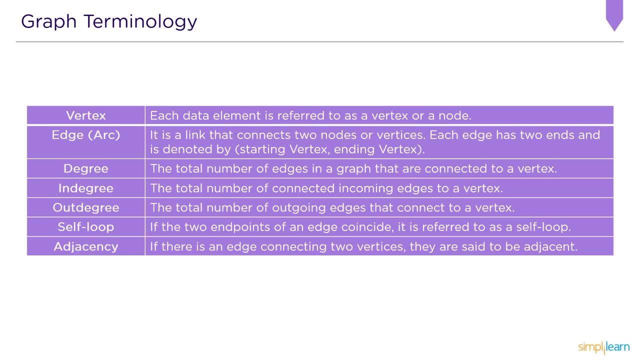 Next we will go over edge graph terminology. It is a connection between two nodes or vertices. Each edge has two ends, denoted by starting vertex and ending vertex. The number of edges in a graph connected to a vertex is then defined as a degree. 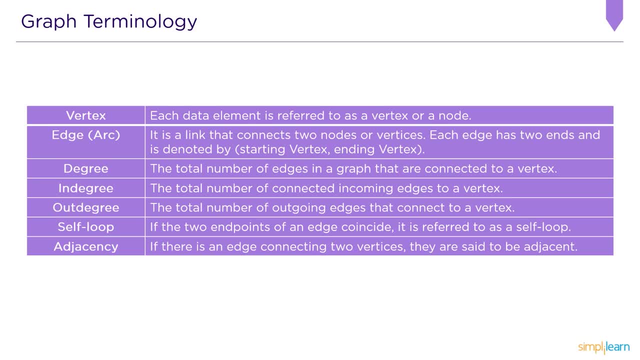 The total number of connected incoming degrees to a vertex is defined as indegree, while the number of outgoing edges that connect to a vertex is defined as outdegree. Then there's a self loop, which is defined as if the two endpoints of an edge coincide. 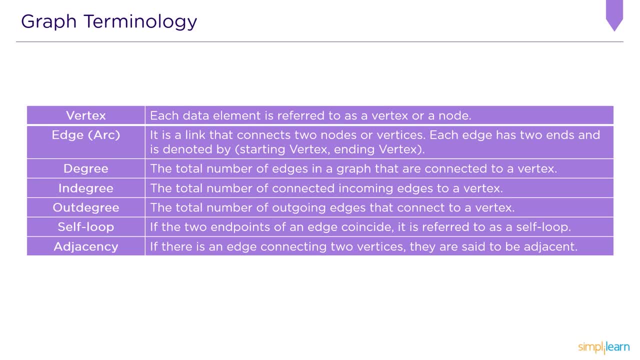 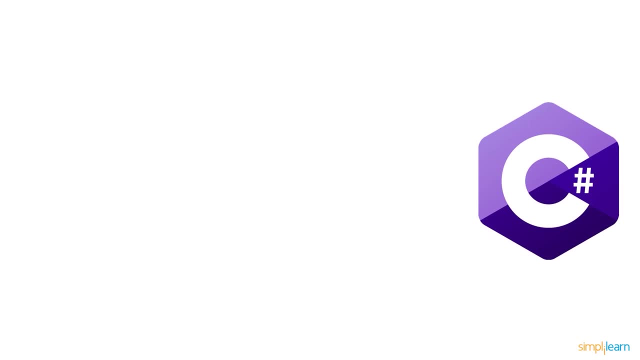 it is referred as a self loop. Finally, we have an adjacency stage, which means that if an edge connects with two vertices, they are adjacent. In this tutorial also covers the graph traversal, which has two types of tree traversal. So the first one is breadth-first search. 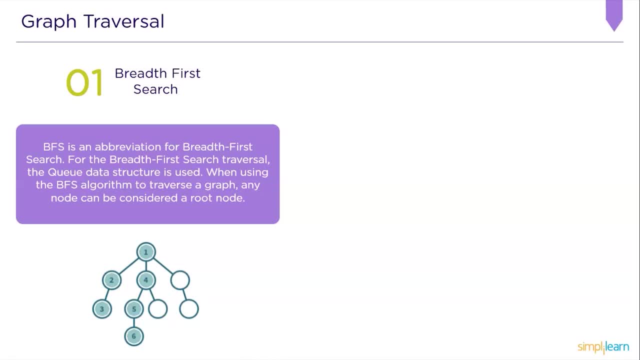 Breadth-first search is the first graph traversal we have, So BFS is an abbreviation for breadth-first search. It is also known as level-order traversal. The Q data structure is used for breadth-first search traversal. Any node can be considered as a reference. 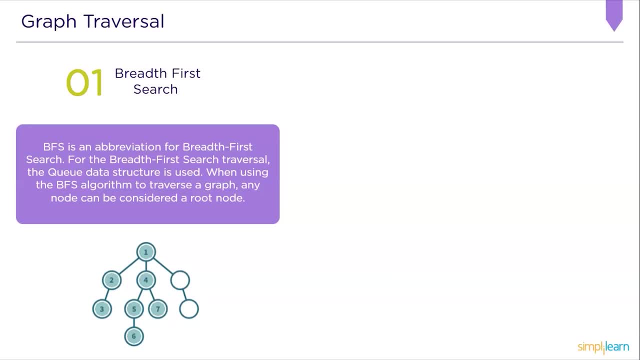 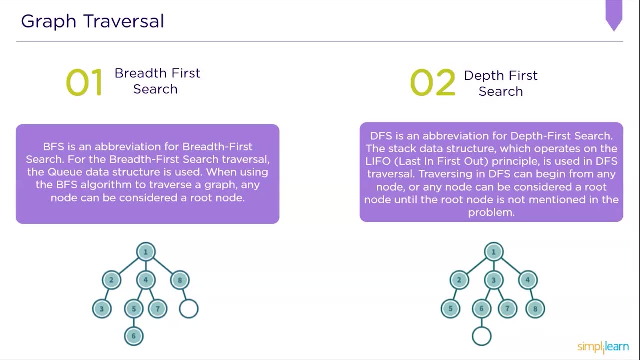 It is defined as a root node when traversing a graph with the BFS algorithm. The second kind of graph traversal is the depth-first search, abbreviated as DFS. In DFS traversal, the stack data structure is used which operates on the LIFO or last. 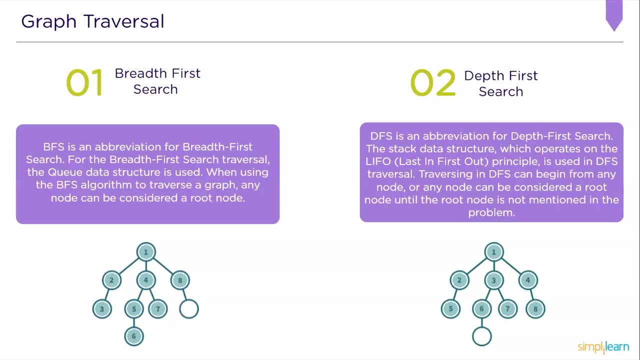 in first start principle, The DFS traversing can begin at any node and any node can be considered as a root node until a root node is not mentioned in the problem. Let's look at the co-traversal of the BFS and DFS graph traversals. 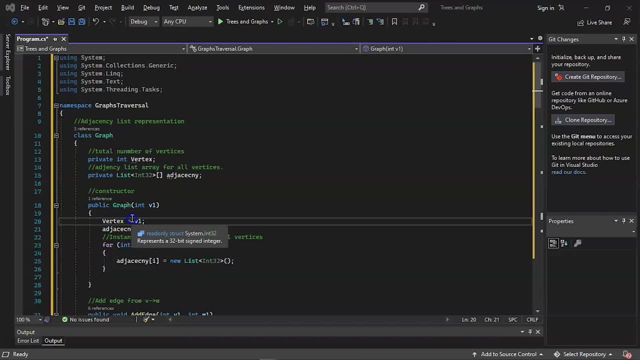 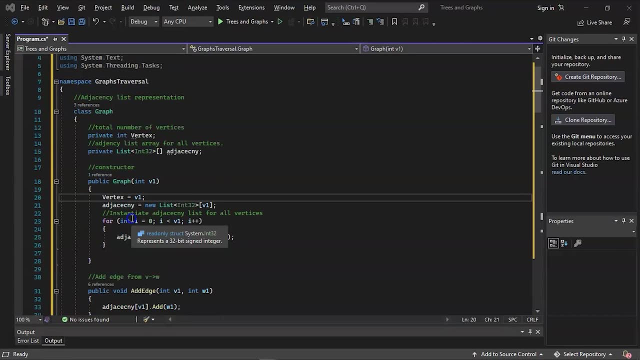 In this program We define namespaces as graph traversal, Then define a class name as graph, We define the vertex variable for the graph's vertex And finally we define the adjacency list array for all vertices. After that we have graph function object, native code with v1 vertex in the parameter. 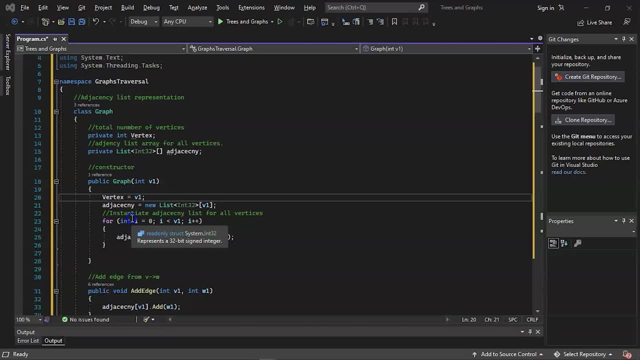 where we assign v1 to the vertex vertex and assign v1 vertices to our adjacency, Then instantiate adjacency list for all vertices. After that we have a loop from 0 to v 1 vertices where we assign the vertices to list of adjacency. 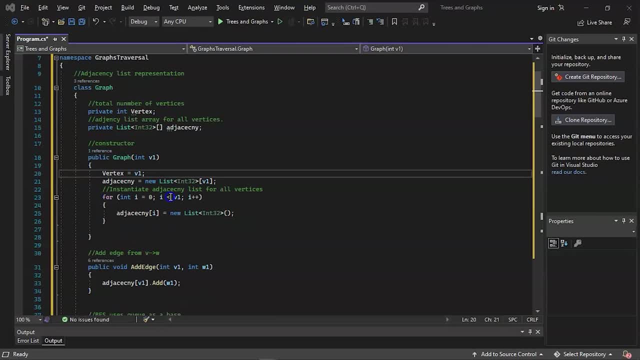 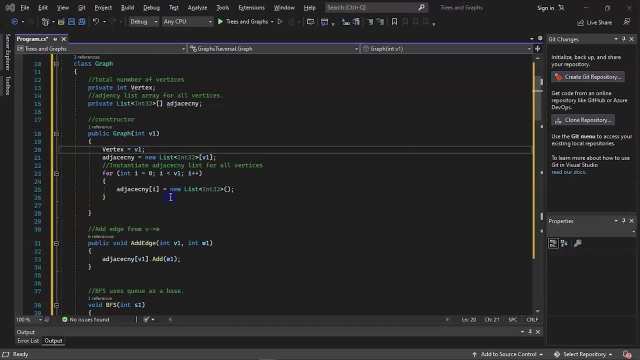 After that we added edge v1 to w1 to the adjacency list. Following that, we define BFS traversal in a parameterized source variable s1, in which we declared an array as a visited boolean data value. Then, as we know, we traverse the breadth first search with Queue data structure and if the 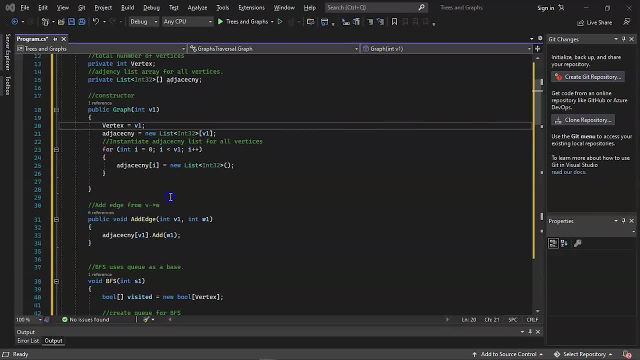 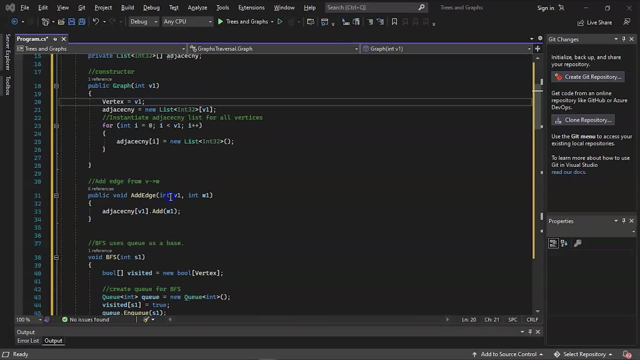 source node is in the visited array. we enqueue the source node to the queue, Then a while loop through all the nodes in the queue And if the queue is not empty, we will dequeue or remove a vertex from the queue and print it. 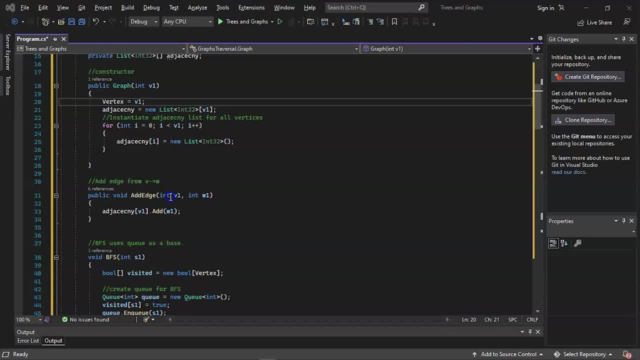 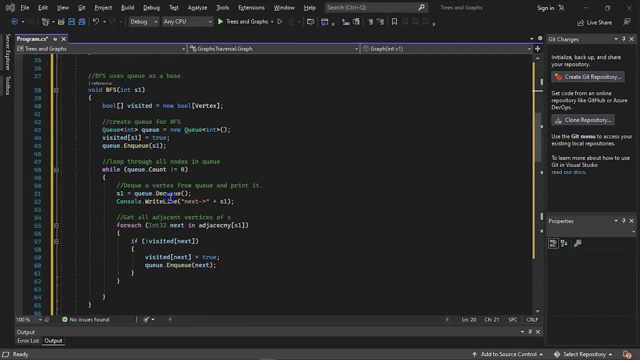 And then we use for each loop to get all adjacent vertices of S1.. After traversing the BFS, we will now traverse the depth. first search in the graph. As we know, stack data structures are used to traverse DFS. So we created a stack with source node as S1 and push the first node as the source node. 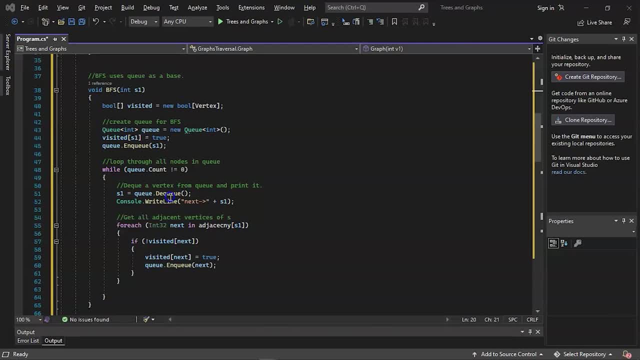 itself. Then we have a while loop that goes through all nodes in the stack And if the stack is not empty, we pop or remove a vertex from it and print it And then we use for each loop to get all the adjacent vertices of S1.. 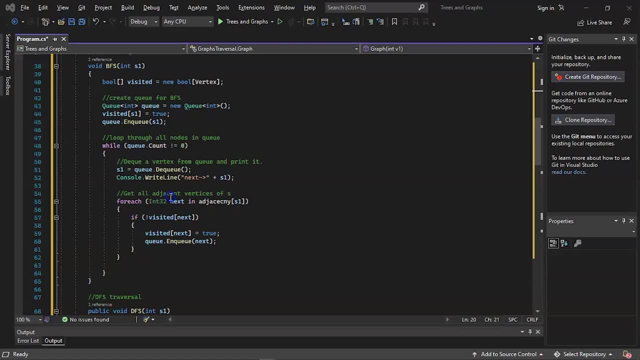 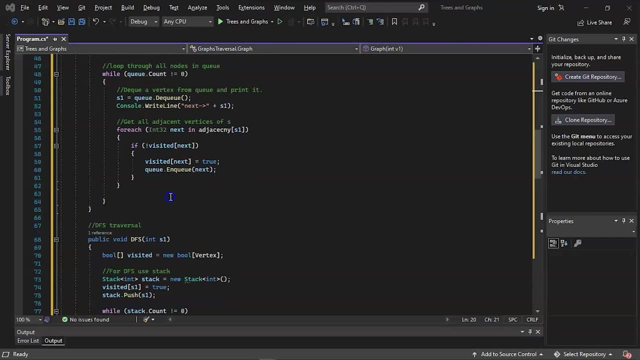 After that we have a for loop that will run up to the last vertex in the graph and start printing all the elements in the adjacency matrix list. Finally, in the main function we have a graph where we call the edge function and add edges. 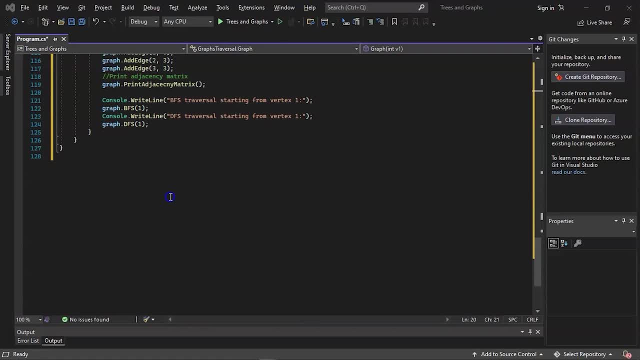 to the graph, And then we print the adjacency matrix And finally we print the breadth function And finally we have the depth first search and depth first search, starting from vertex one. Now let's quickly try to execute the program and see the output. 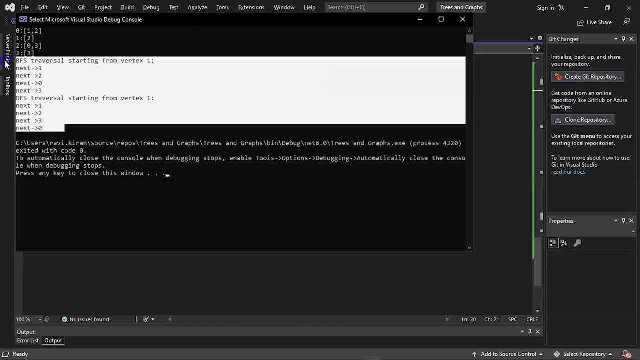 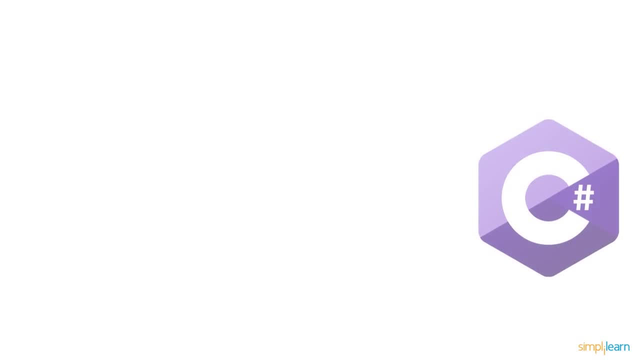 So there you go: The code got successfully executed and you have both BFS and DFS traversals from vertex one. Now let's quickly get back to the PPT. Following our understanding of graph traversal, we will look at some graph representations in C sharp. 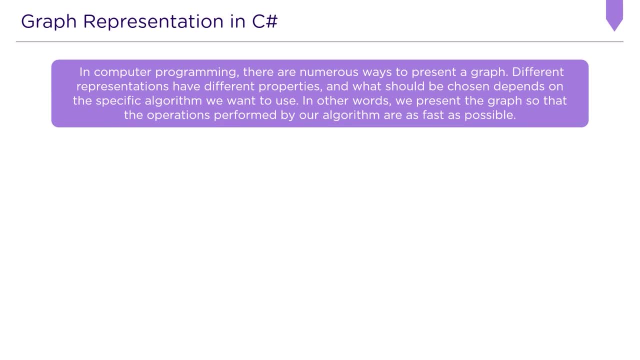 In computer programming, there are numerous way to represent graph. Different representations have different properties, and what should be chosen depends on specific algorithm we want to use. In other words, we present the graph so that the operations performed by our algorithm are fast as possible. 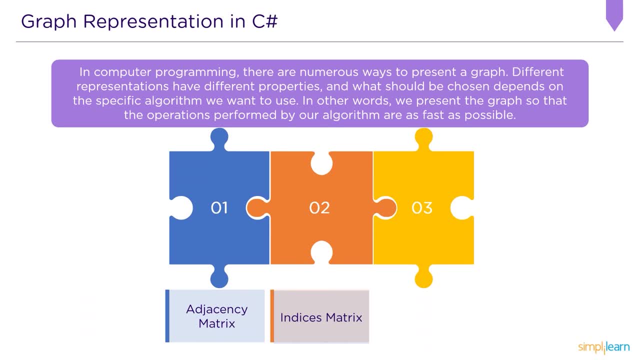 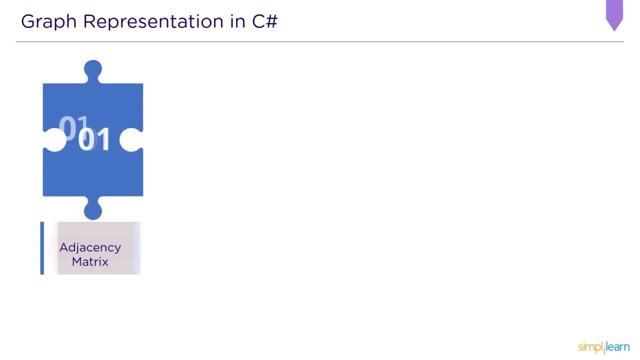 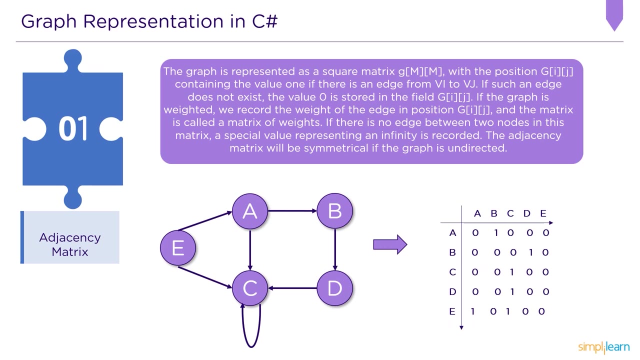 So the first graph representation is an adjacency matrix, followed by an indices matrix and finally an adjacency list. Let us define all three graph representations in greater detail, beginning with the adjacency matrix. The graph is represented as square matrix with the position G, i, j containing the value. 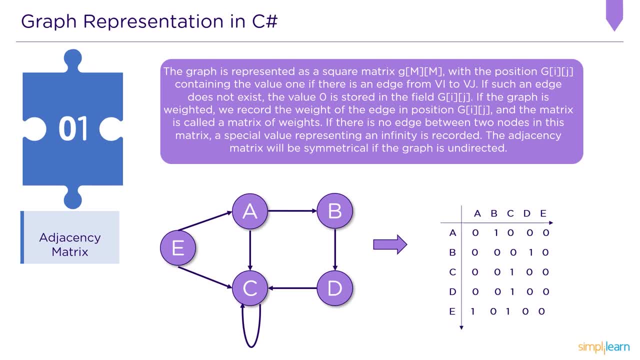 of 1.. if there is an edge from Vi to vj, If such an edge does not exist, the value 0 is stored in the field gij. If the graph is weighted, we record the weight of the edge and in the position gij, and the matrix is called a matrix. 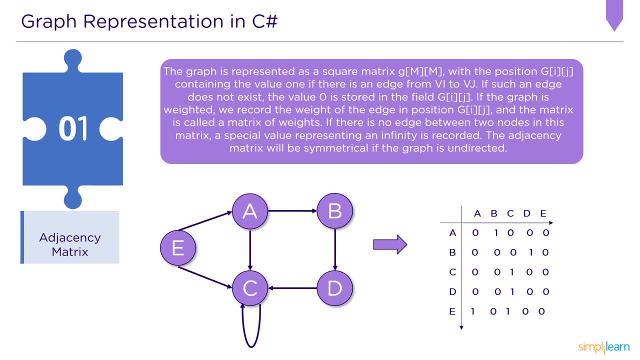 of weights. If there is no edge between two nodes, this matrix- a special value representing the infinity- is recorded. The adjacency matrix will be symmetrical if the graph is undirected. The next graph representation is an indexes matrix. A graph can be represented using an. 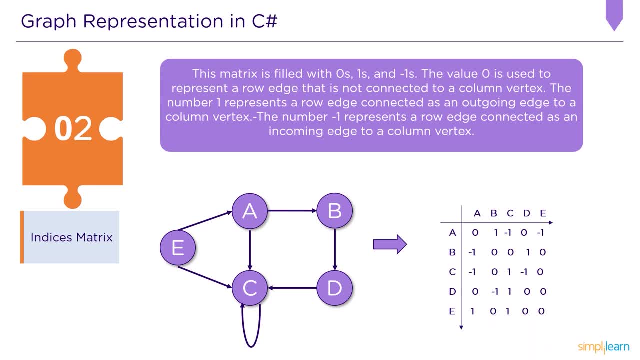 incidence matrix with the following dimensions: This matrix is filled with zeros ones and minus ones. The value 0 is used to represent a row edge that is not connected to a column vertex. The number 1 represents a row edge connected as an outgoing edge to a column vertex. The number: 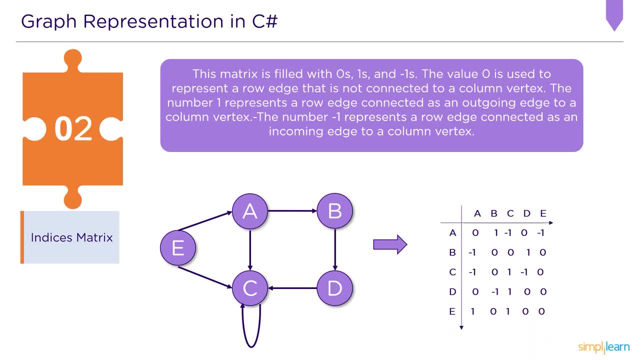 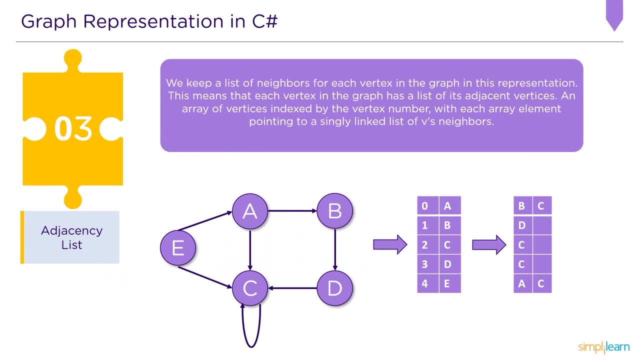 minus 1 represents a row edge connected as incoming edge to a column vertex. The last graph representation is the adjacency list defined as. in this representation we keep a list of neighbors For each vertex in the graph. this means that each vertex in the graph has a list of adjacency. 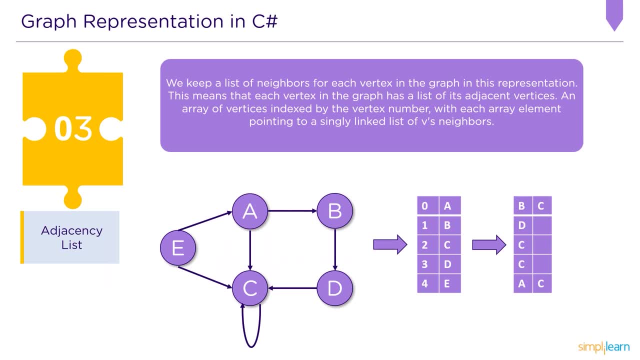 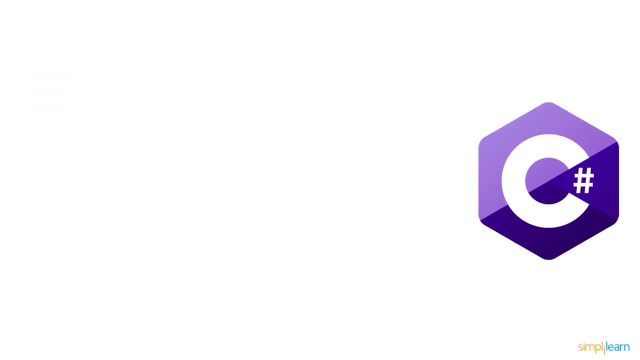 vertices: An array of vertices indexed by the vertex number, with each array element pointing to the singly linked list of these neighbors. Finally, in this tutorial we will look at the real world examples of graph data structures. So here are the six real life examples of graphs. 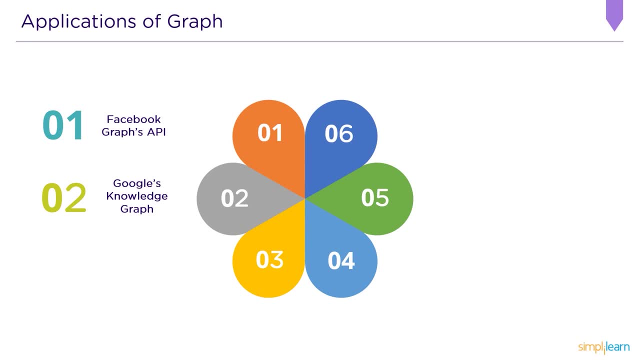 We have Facebook graph API and we have Google knowledge depth. We have Yelp's local graph, we have Path-Optimization-Algorithm and, finally, we have Google Map Platform and, finally, Flight Network. Now let us see a little more detail on all these applications. 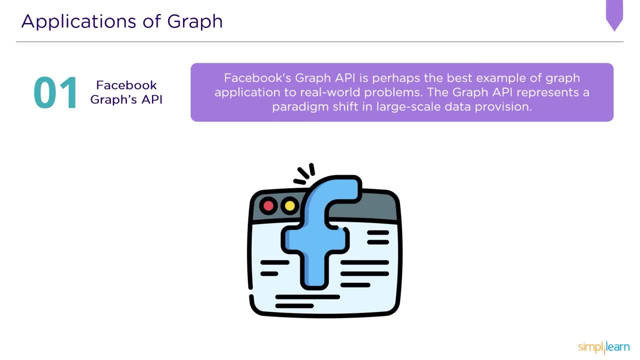 Facebook graph API. This graph is both predefined as CHARGE and specific to apps. they, too, have specific characteristics and are generally based on the self-assessment method for occasional, automatically related events. following that are often referred to as metadata nichts Knowledge Graph. This graph is product-based and it is defined as a graph representation of knowledge that.